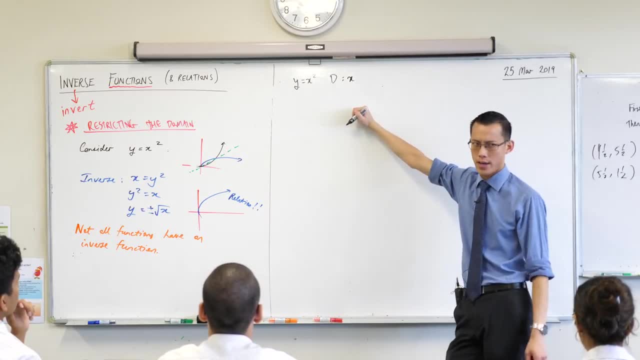 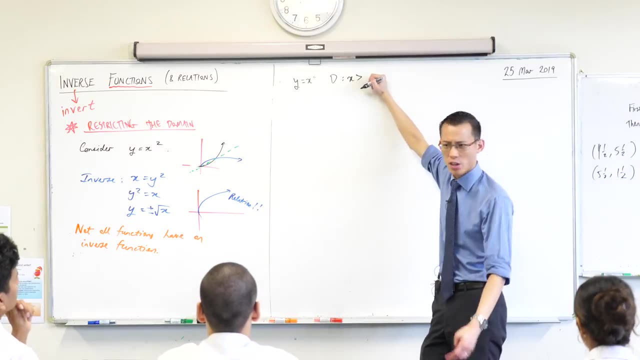 Well, how would I say? this is an inequality. What part of the graph have I got? What values of x Greater than Do you reckon I can include 0?? I think including 0 is okay right, Because, remember, what I don't want to have is any double ups, right? 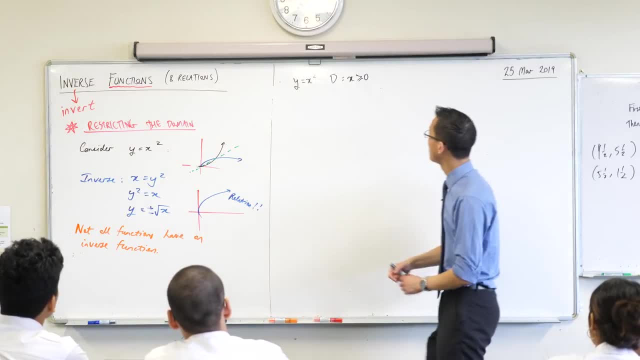 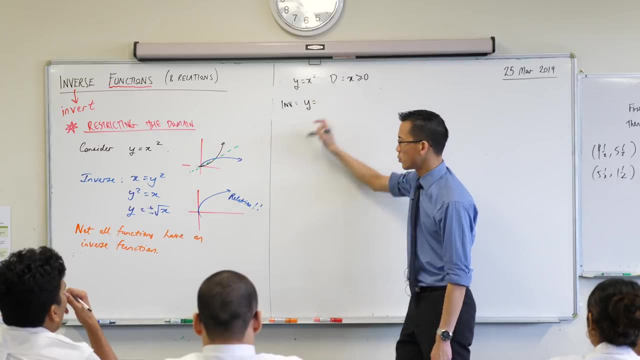 But at x equals 0, you don't have a double up, It's just right there at one spot, right? So if I take this, then the inverse will become y equals. Well, you only get the top part. See that. 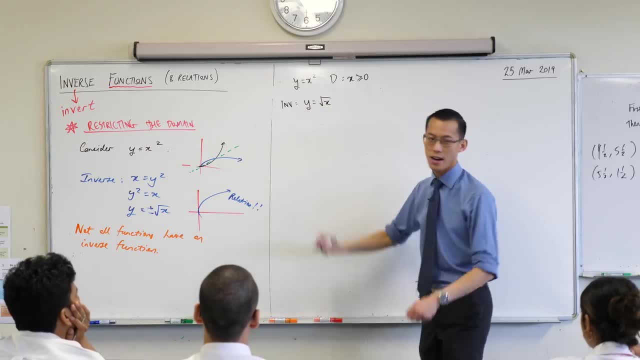 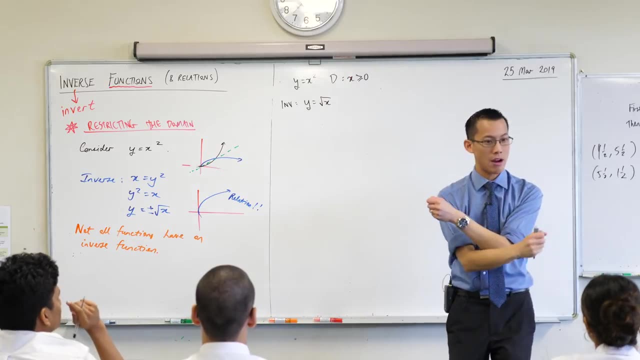 You have to disregard the negative bit, right? So you get this guy. Now, the domain x is greater than or equals 0.. Remember, when we went from a function to its inverse, We swapped everything, right, We swapped. every x becomes a y, every y becomes an x. 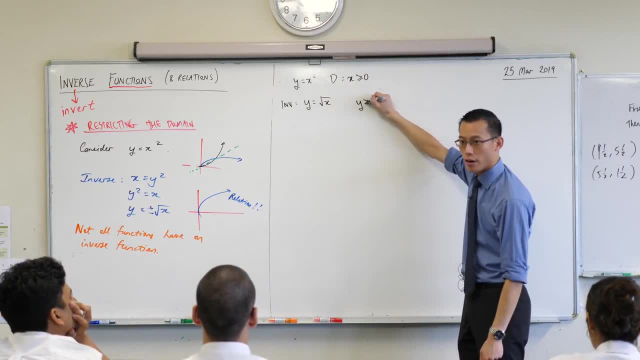 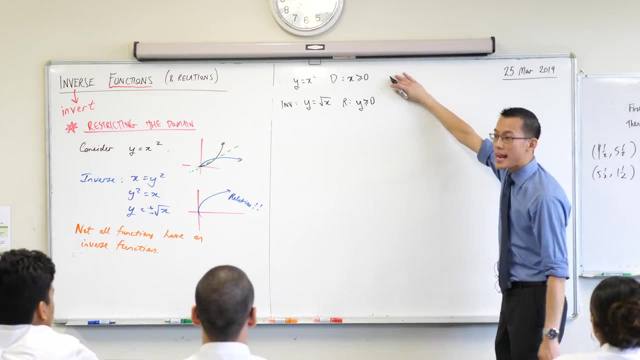 Well, when you swap this, you get a y is greater than or equals 0. That's not domain anymore at all. What is that? That's range, right. So this is actually really important. The domain of your original becomes the range of your inverse. 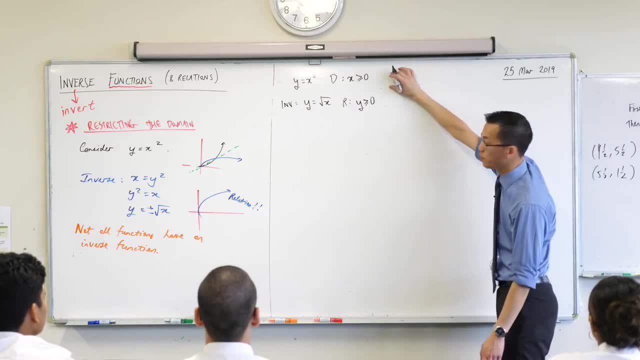 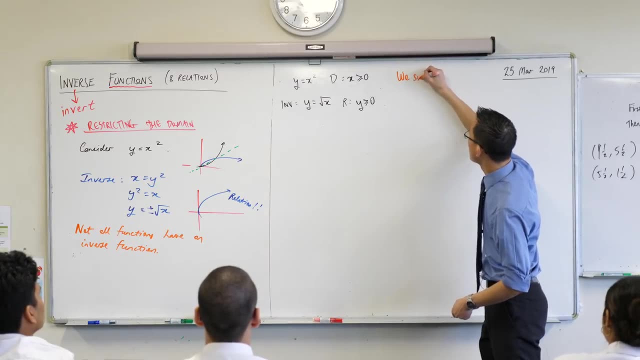 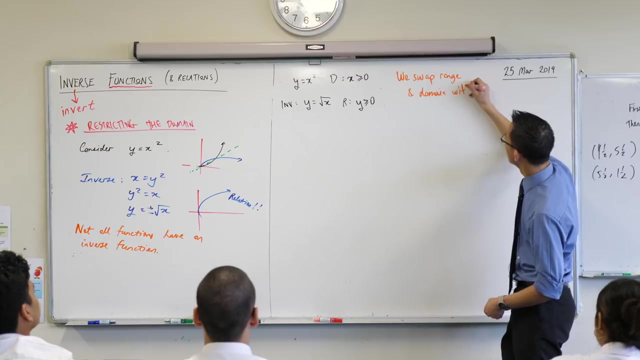 And the, if we cared about it, the range of your original becomes the domain of your inverse. That's actually worth writing down. When we swap x's and y's, we swap range and domain as well. So what we're doing is we're making it a very simple thing. 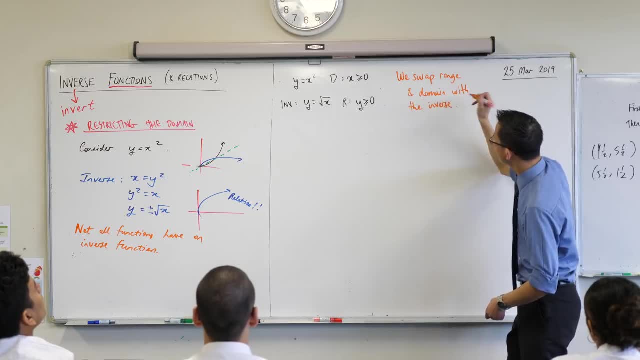 So what we're doing is we're making it a very simple thing. So we're making it a very simple thing. So what we're doing is we're making it a very simple thing. Okay, now just a really small sub-note, right? 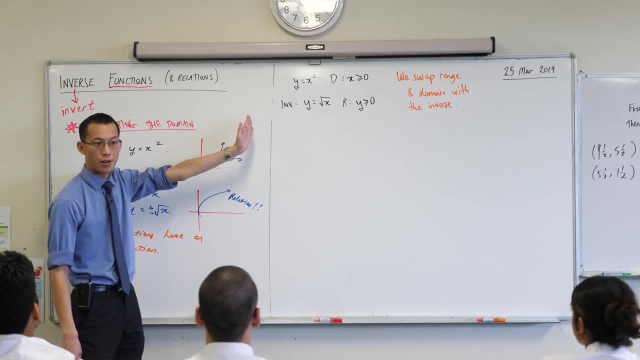 You notice, over here I was like I just chose a part, We just chose this part over here, right? Would anyone like to suggest to me: why didn't we- You don't have to draw this, by the way- Why didn't we pick the other part? 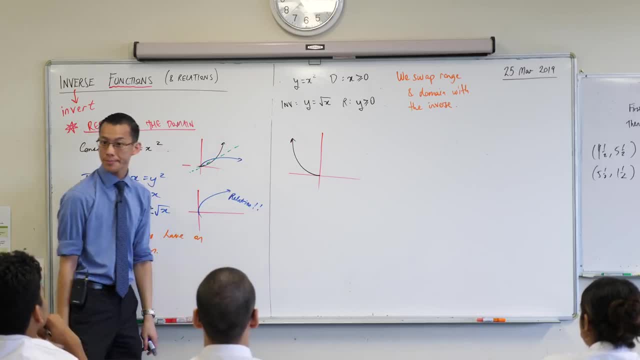 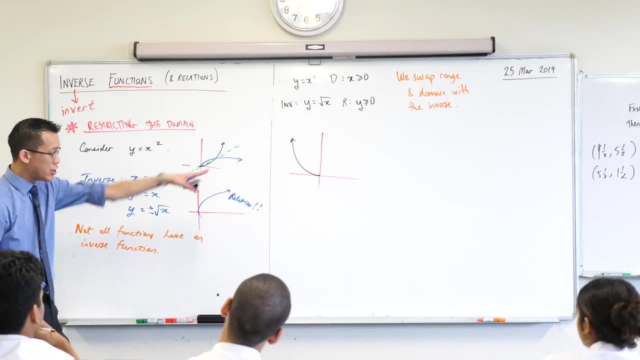 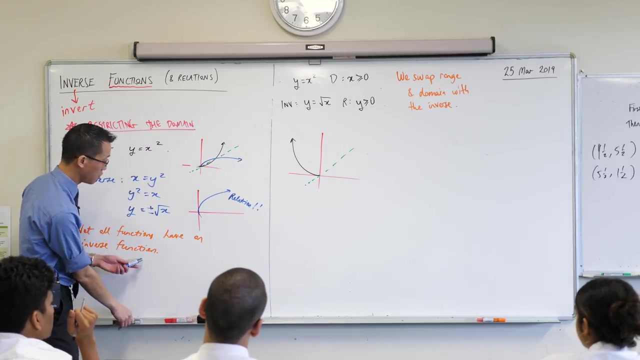 Like this part. over here there's another restriction. What's the domain of this graph? Okay, Okay, Okay. over here, x is the less than or equal to 0. right now you can take that and, just like before, you can put on: y equals X and you can reflect it across, you will. 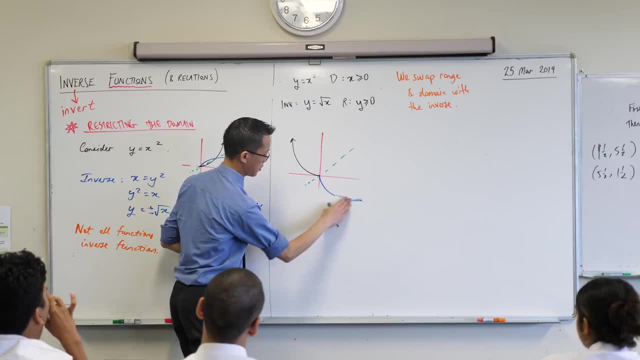 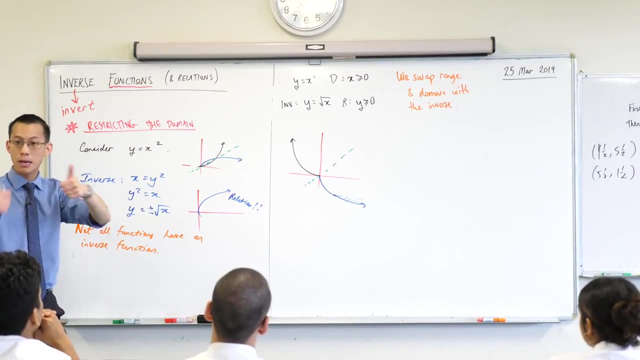 get this shape over here. that's sort of too far, sorry, there we go, so you're still gonna get like: is that? is that an inverse function? the blue graph thumbs up right, so why don't we do that? why do you think we will do this rather than? 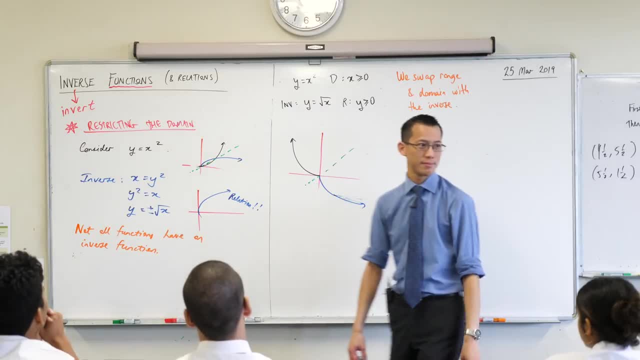 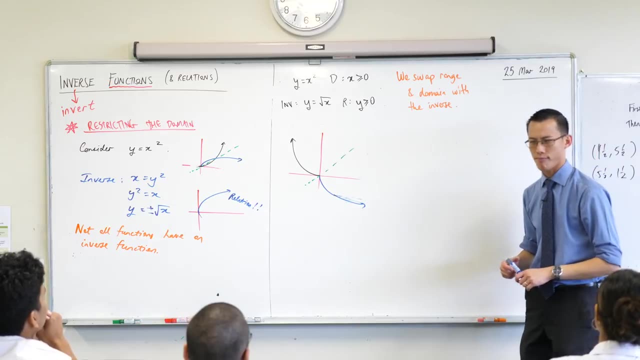 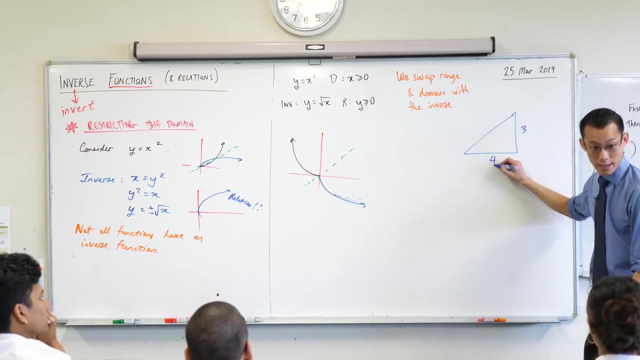 this then you take is: when did you first start using square roots? what topic was it in, do you remember? hmm, way before indices, it was actually Pythagoras, right, because you'd say: oh, if you know what this side is and you know what this side is, then you'd say: this is the square root of this, plus this. you're like: 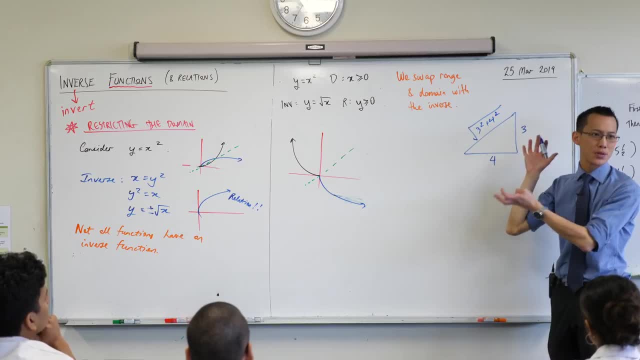 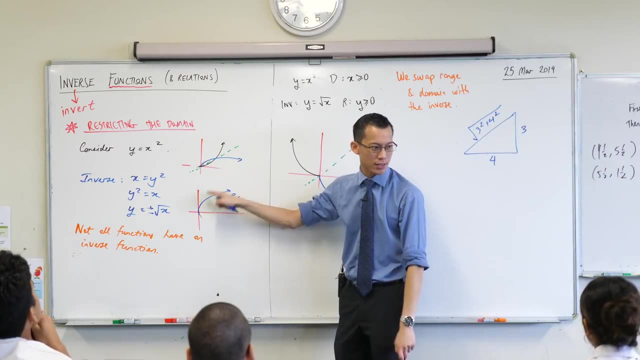 what do you want? I need to know what square roots are right. but in the context of measuring triangles, the only thing that makes sense is a triangle positive value. you want to get things above the axis. those are positive values you're like: well, these are. I mean, I could take them, but what's the point? 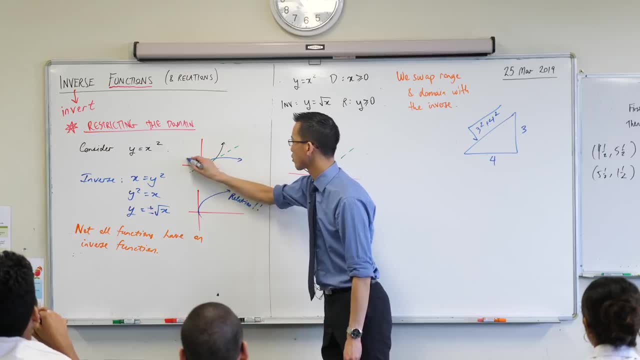 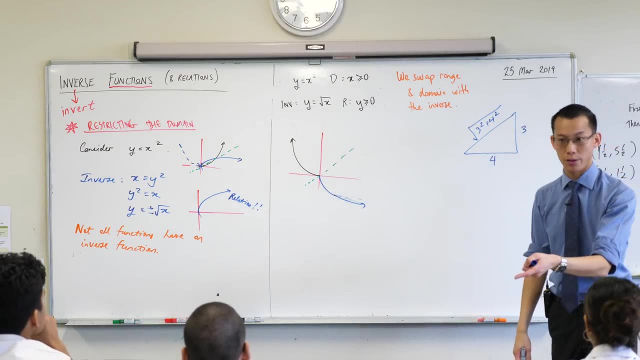 okay, now the real issue is: uh, if I put the rest of the graph back on, the real issue is that guy there. see how it turns around. that's the issue. right, the two graphs that we started with? 3x minus 1, I think, and what was it? X cubed plus 2, the 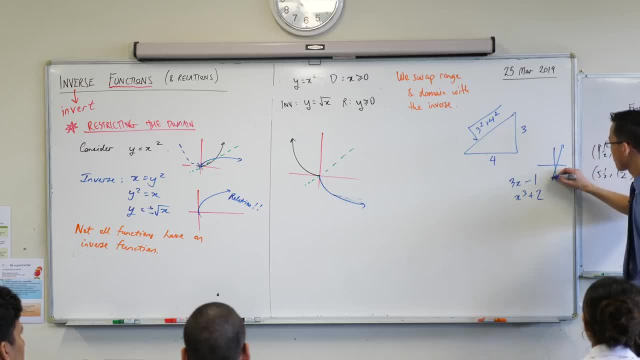 reason I gave you these two is because neither of them turns. did you notice that you can go back to where you drew these on your page like there's no turning point? and so these are both. think back to our classifying functions. do you remember when we did that one many business, all that kind of thing. 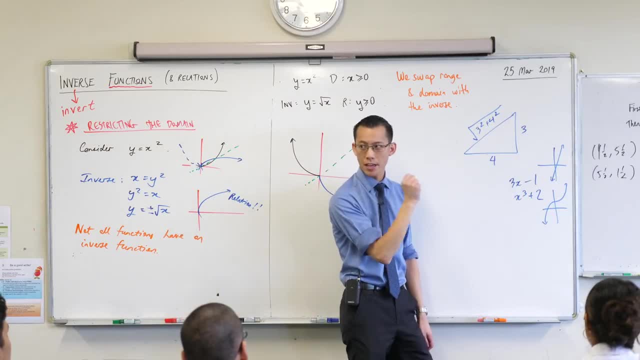 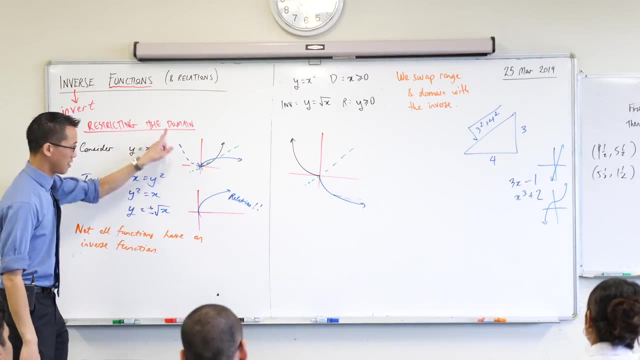 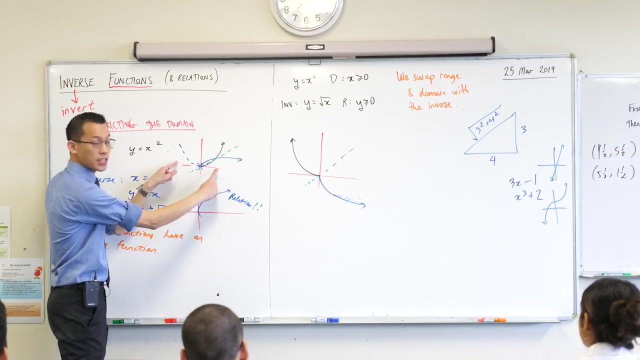 right. what kinds of functions are these? think about them. these are both one to one. that's why I deliberately gave it you. I just didn't tell you right. but this guy over here, the original y equals x. squared is not one to one, is it? which one is it? it's many to one, many different x values. oh, 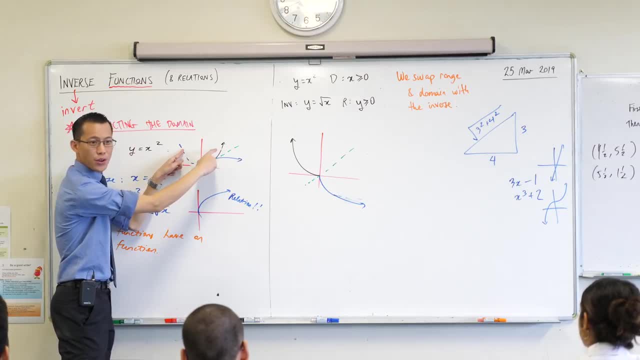 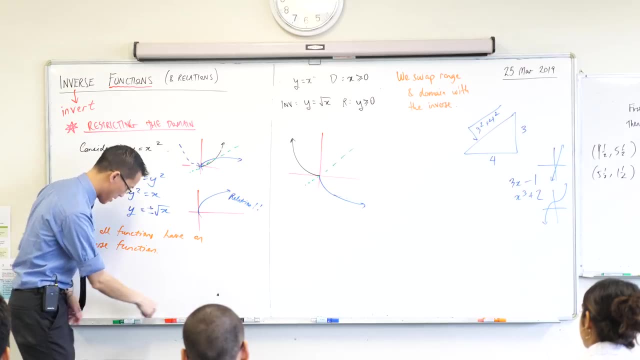 will give you the same y-value, right? So the problem with having a many-to-one is that when you swap everything around, you're swapping the many and the one. you get a one-to-many- this guy, which is not a function anymore, right? 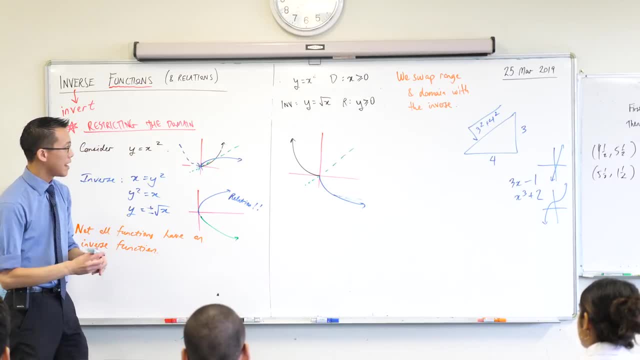 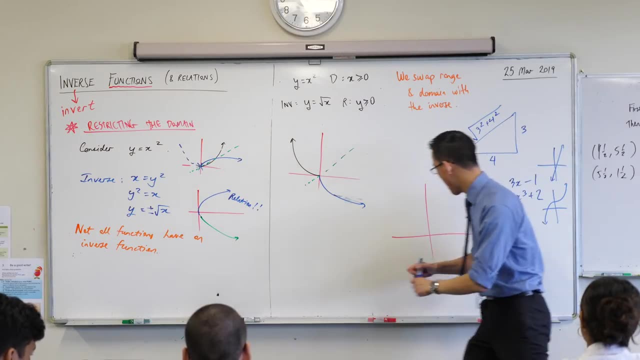 So that's why we have to learn to restrict the domain. Now. if, for example, I'm not even going to worry about the numbers, I'm just going to draw a picture for you, right? If, for example, I gave you a graph like this: 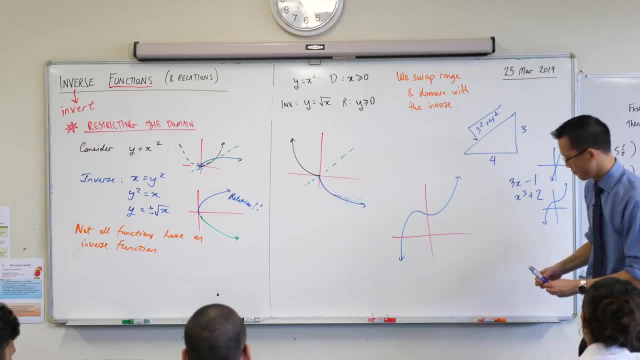 when I take this and do the inverse of it, right? What will be the problem? Well, you know how we look for the vertical line test over here, right? When you're thinking about inverses, everything swaps. Vertical isn't vertical anymore, it's now going to be horizontal, right? 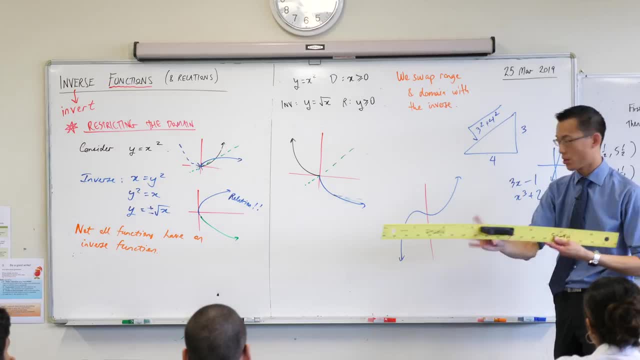 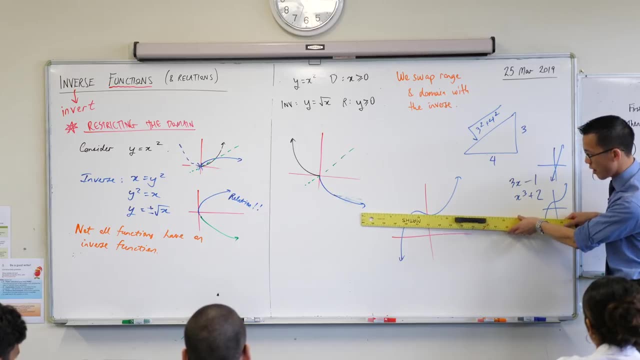 If you swap x and y, this vertical line becomes horizontal. So if I put a horizontal line against this right, Have a look. Is there a place where it fails? And the answer is yes, Like anywhere up in here, you're in trouble, right? 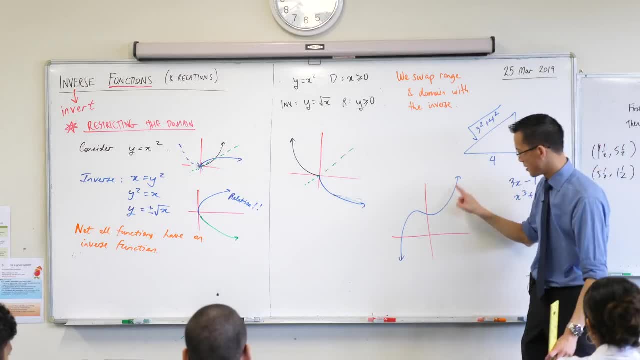 So if I swap, If I swap this thing around, you will not get a function because this part here, once I reflect it over, will fail the vertical line test. Does that make sense? So I need to restrict the domain. So if, for example, let's call this: 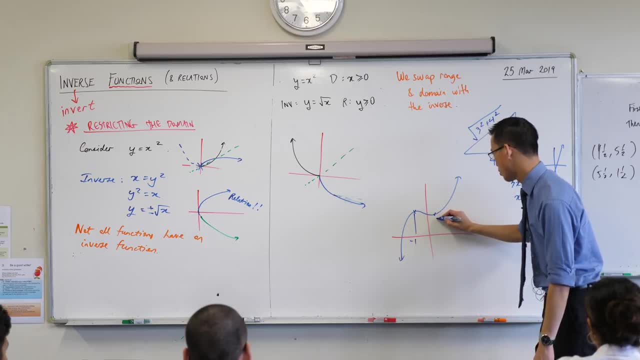 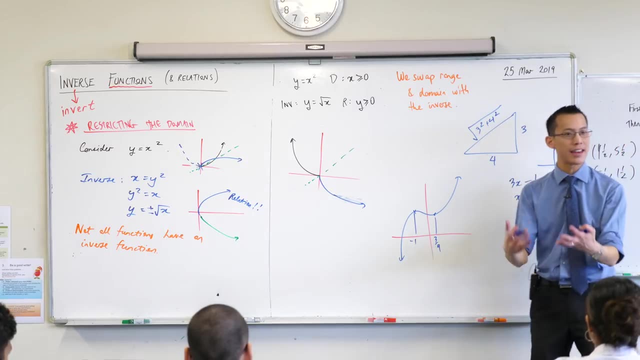 Let's just give it a value. Let's call that negative one right there And let's call this: I don't know, that looks like three quarters or something like that. okay, I could take sections of this. Can someone give me an example of a restricted domain? 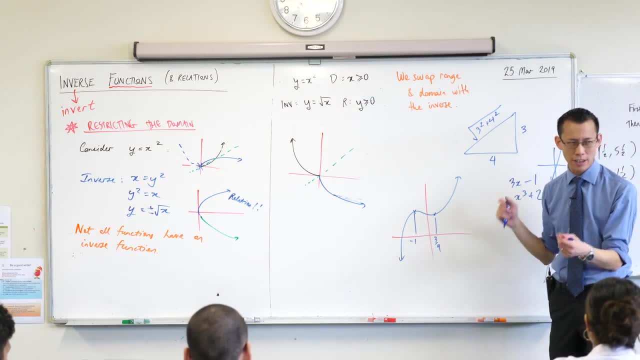 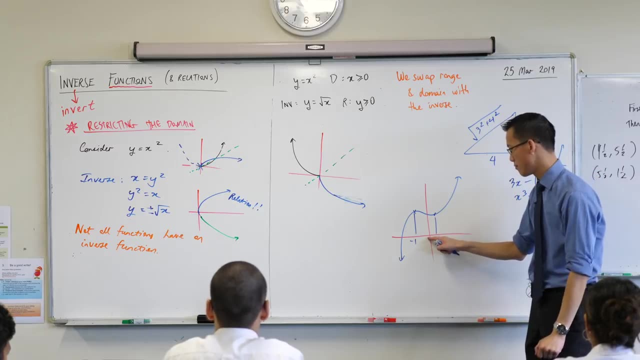 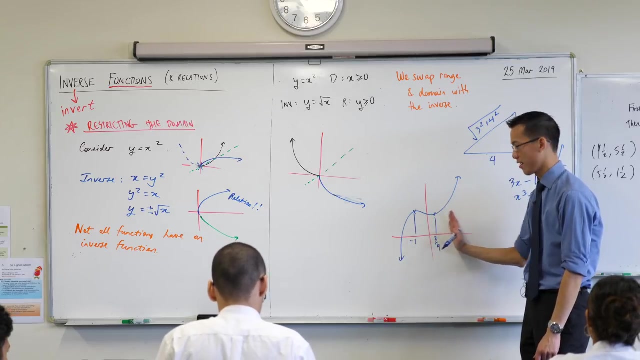 which, if I took the other side, if I took the inverse, it would give me a function. Someone give me an example. What are you thinking, Rassan? Zero to where? Zero to where Minus two? To the left or the right? 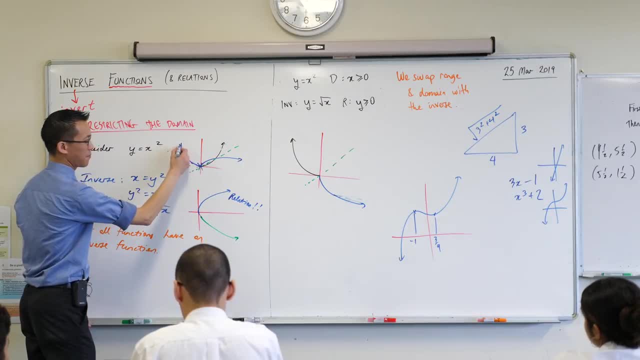 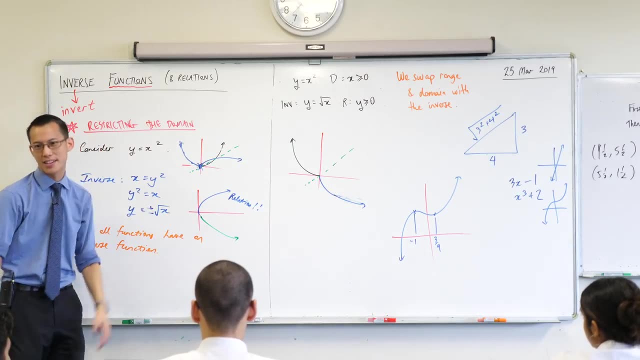 Think, right, Come back over here, Look at this original guy. right, I said okay to the right is okay, To the left is okay. It's this point where it turns that it's the problem, right? So, for example, let's just hide. 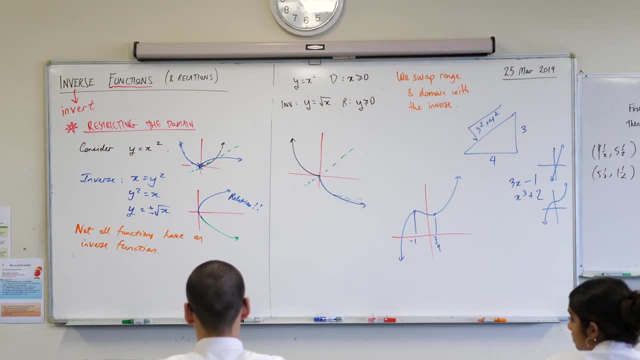 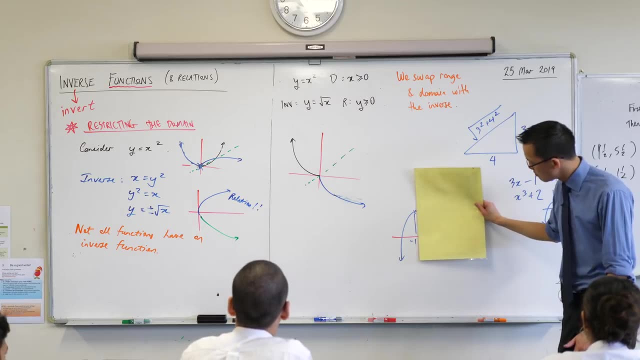 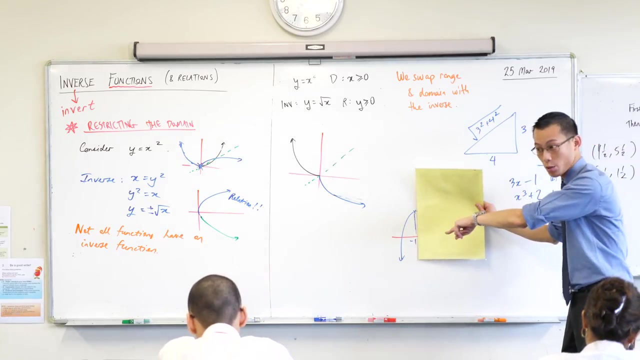 This will do. I need something big One to one right. See that section there. If you did the reflection, that part would be okay, right, It would. It fails, Sorry. It passes the horizontal line test. So when you flip it over, it'll pass the vertical line test, right. 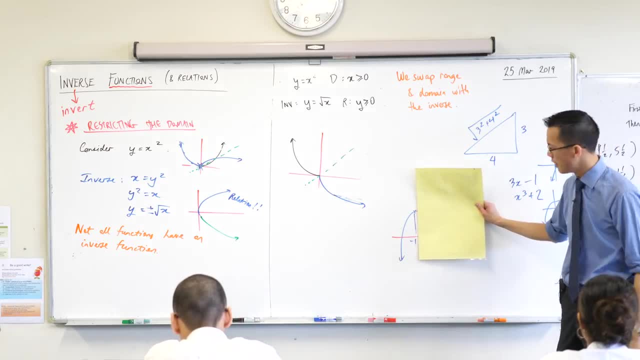 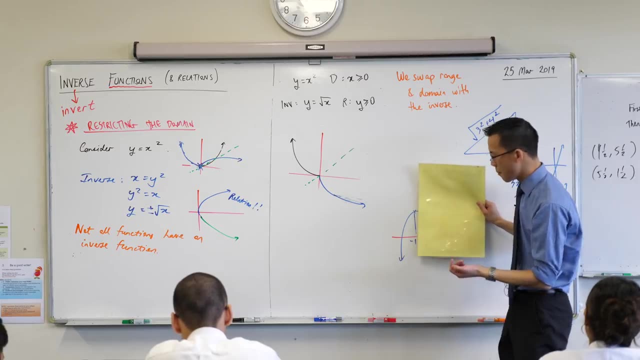 So this part's okay. How would you state that inequality? that domain Minus one to the third of four, Yeah, X is less than negative, one or equal to is five. right, But that's not the only section that works, right. 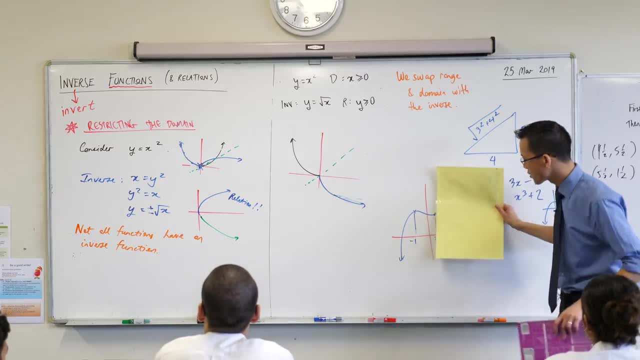 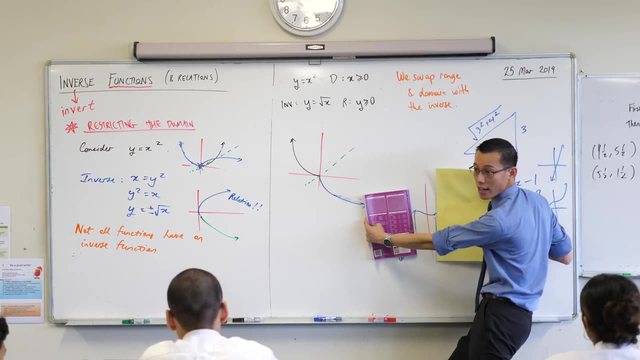 I need another thing to hold up. Sorry, There we go. So if I take this section here, See that spot there. You see, this little section here is one to one, right? So if you did that reflection, it's going to be fine, right? 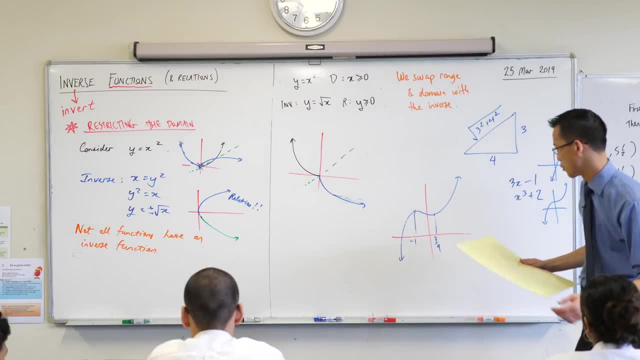 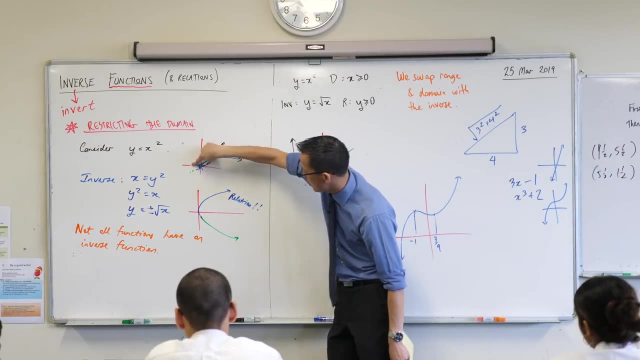 There's one last section. Can you see it? Can you tell me what it is Now that I've, like, ruined what I've written on the board by here, Yeah, Over here. right, This part here looks just like the part that we restricted for the X squared graph, right? 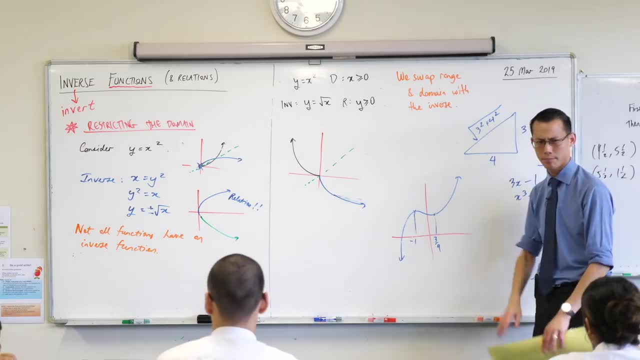 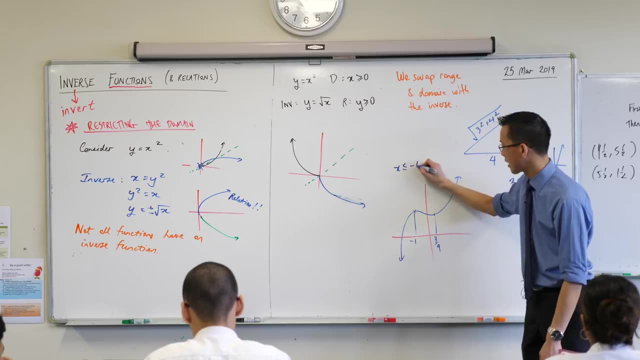 So you can actually pick any of these bits and you'll get an inverse function out of it. Does that make sense? So I'm going to write those answers for you, just so you know. right, X is less than negative one. That would give me an inverse function. 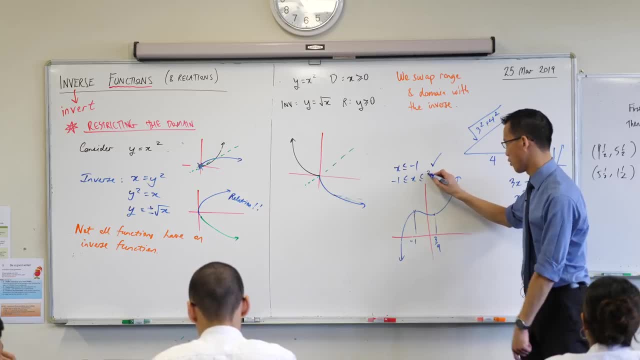 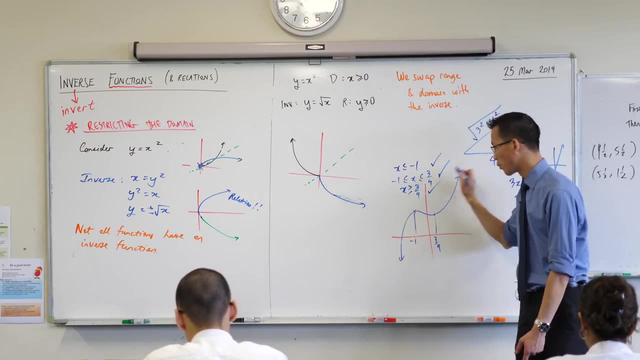 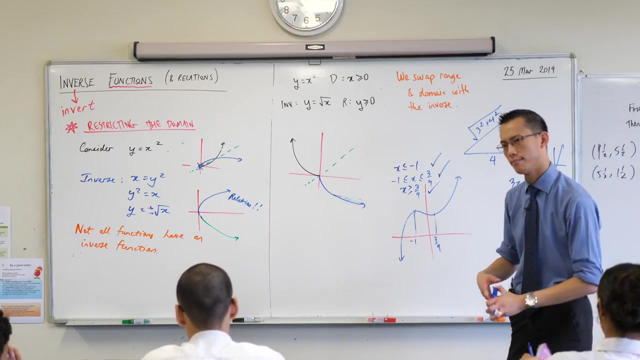 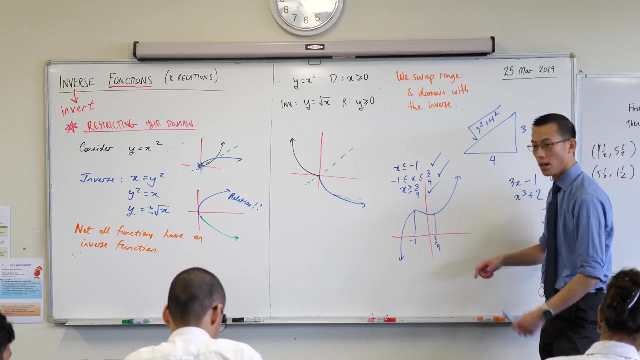 Between negative one and three over four, That would give me an inverse function. Or To the right of three over four, That would also give me an inverse function. Say it again, This one over here You mean like an interval notation. 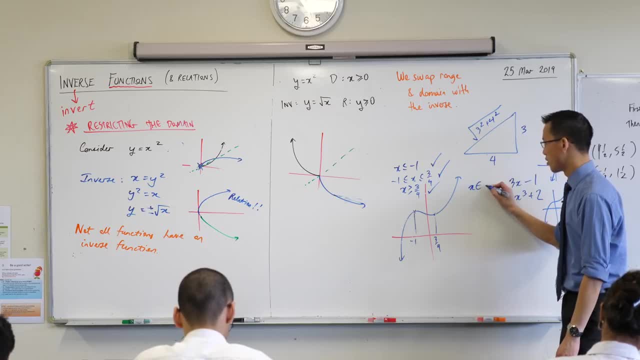 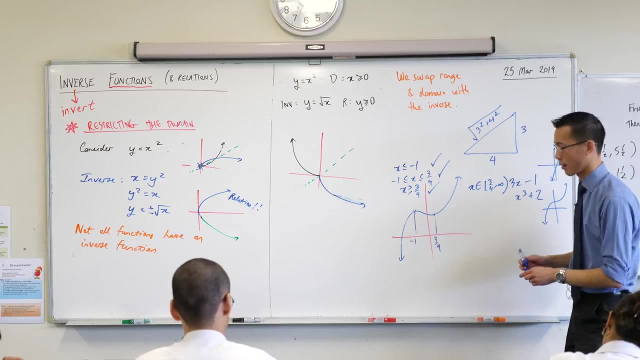 You could- I mean exactly the same- as this would be to write that X belongs to three quarters all the way to infinity. You could write it like that if you want, but they're exactly the same thing, Okay. Okay, All right. 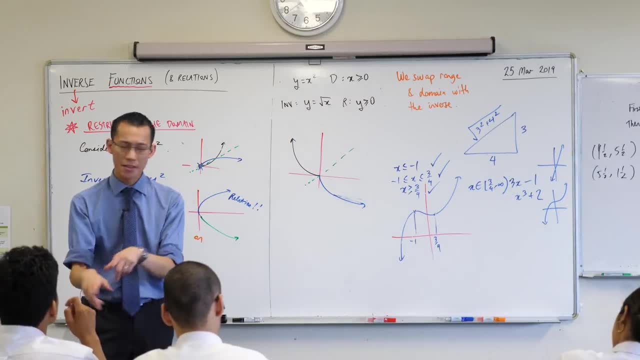 So in questions seven, eight, nine and ten, they're going to ask you about this right. They're going to ask about: well, tell me about this mutual inverse thing. Can you show that this really is the inverse by putting one into the other?